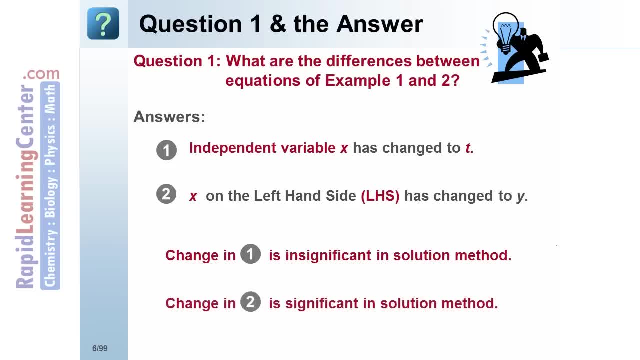 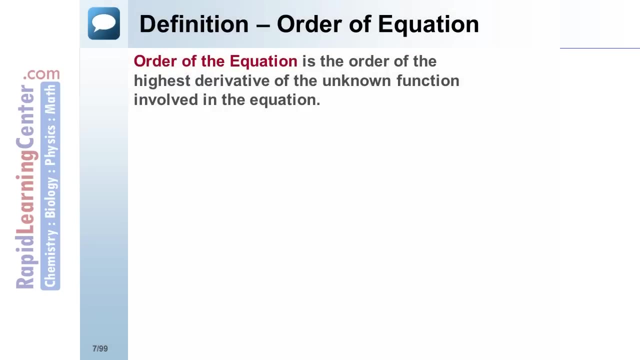 The change in 1 is insignificant in the solution method, But the change in 2 is significant in the solution method Definition. The order of the equation is the order of the highest derivative of the unknown function involved in the equation, Example 3.. 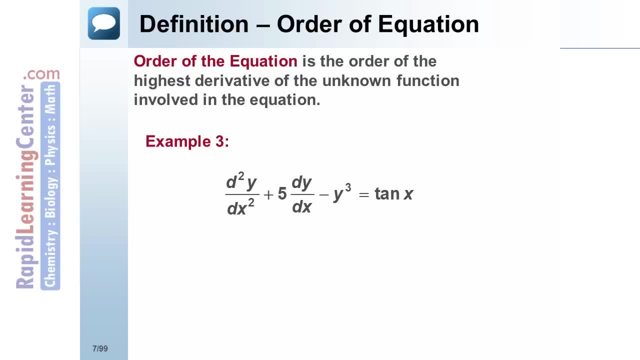 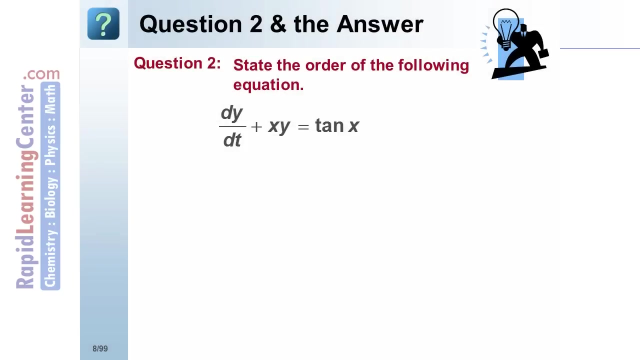 The second derivative of y with respect to x Plus 5 times dy, dx minus y cubed equals tangent of x. This equation is second order Because the highest derivative involved is the second derivative of y. Question 2.. State the order of the following equation: 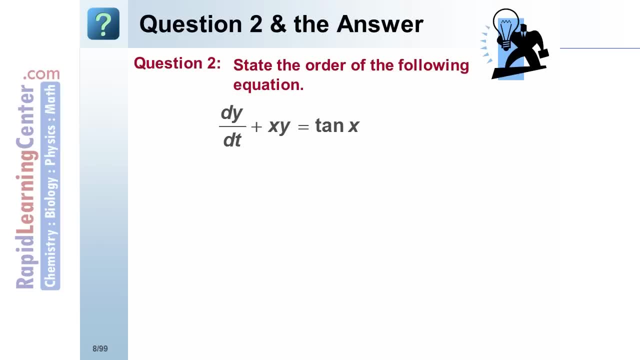 dy dt plus x, y plus 5 times dy dx minus y, cubed equals tangent of x plus x y equals tan x. This is the first order equation, Because the highest derivative involved is of the first order. We will only investigate the first order equation in this tutorial. 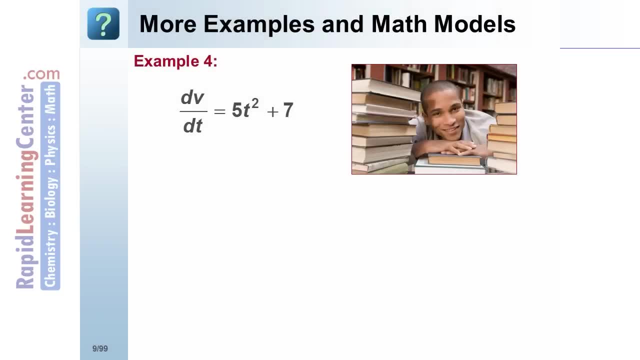 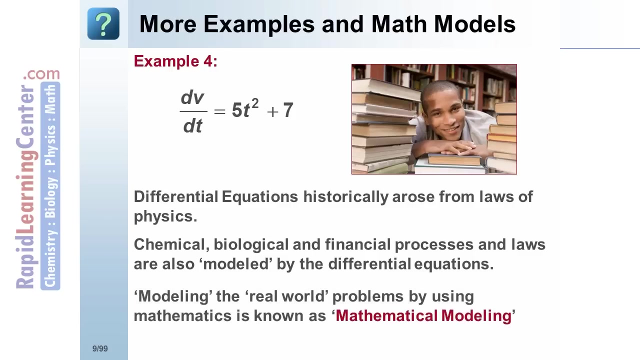 Here's another example of a differential equation. Here's another example of a differential equation. Here's another example of a differential equation. The differential equations historically rose from laws of physics, Chemical, Biological and Financial processes and laws are also modeled by the differential equations. 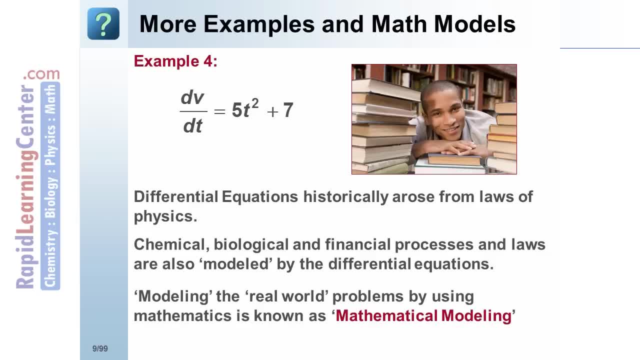 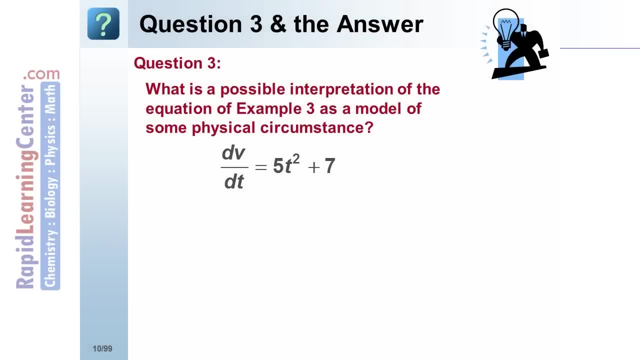 Modeling the real world problem by using mathematics is known as mathematical modeling. Modeling the real world problem is known as mathematical modeling. This worst-case situation costs up to a hundred thousand dollars. Question 3. What is a possible interpretation of the equation of example 3 as a model of some physical circumstance? dv dt equals 5t squared plus 7?. 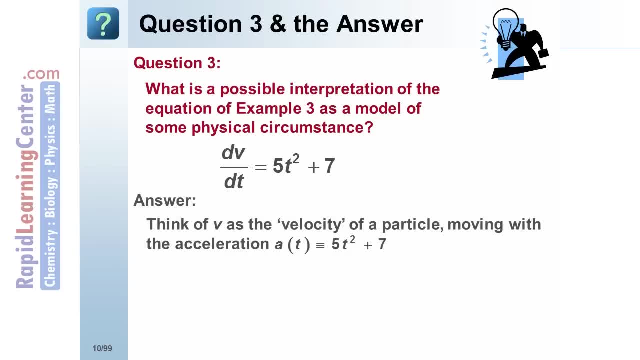 Answer: Think of v as the velocity of a particle moving with the acceleration. a of t equals 5t squared plus 7.. Since a of t equals dv, dt, this gives us our differential equation. Differential equations are often used to predict what will happen in later time, knowing the values of the unknowns initially. 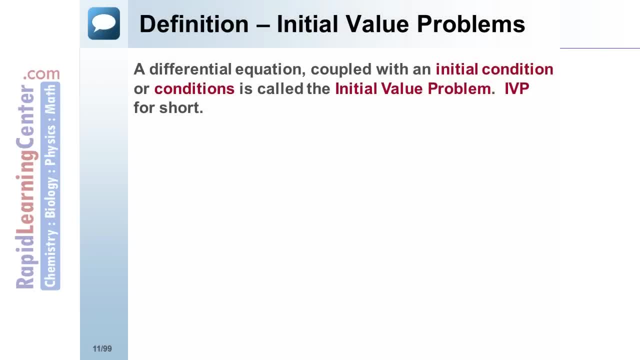 Definition: A differential equation coupled with an initial condition. A differential equation coupled with an initial condition or conditions is called the initial value problem, IVP for short. The equation in example 4,, coupled with the initial condition dv, dt equals 5t squared plus 7, and v of 0 equals 17,, is an example of the IVP. 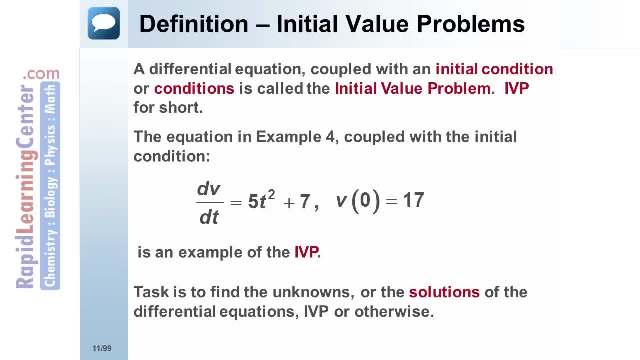 The task is to find the unknowns or the solutions of the differential equation IVP or otherwise Differential equations. 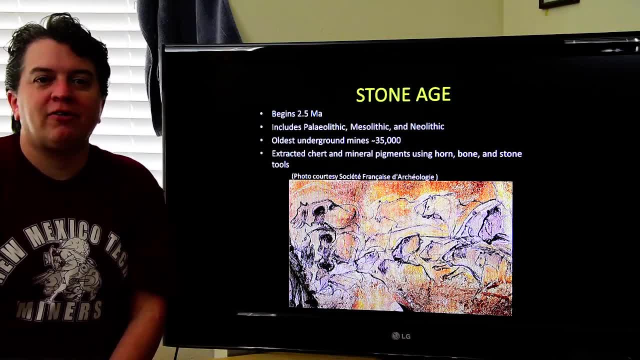 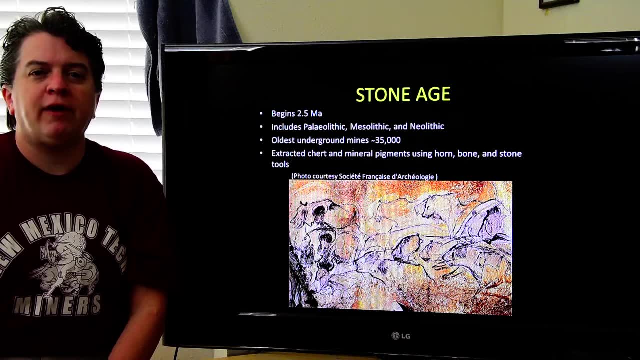 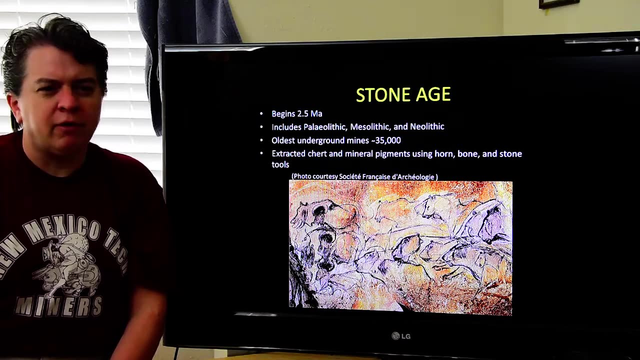 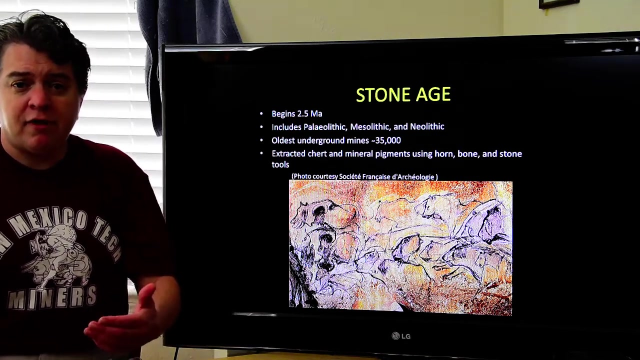 Hi guys, today we're going to talk about mineral resources. We use minerals in all kinds of things every day and never really think about it. Our houses, our cars, our tools, our computers- all this stuff is made with materials that we get out of the ground, And that's the subject. 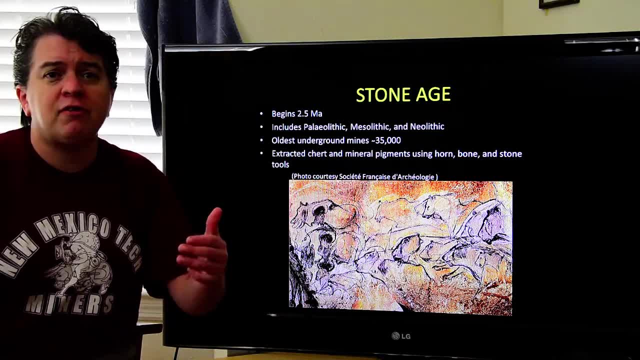 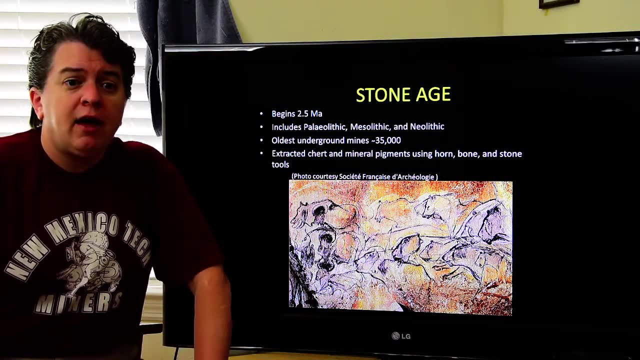 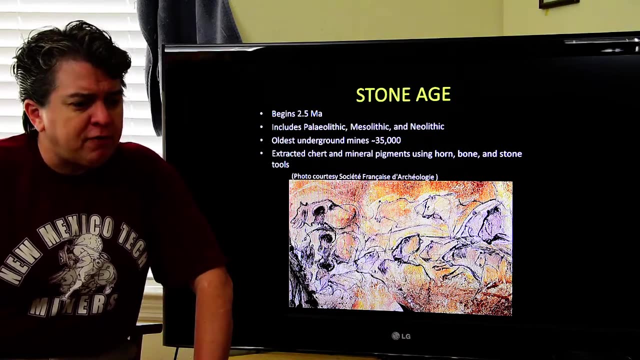 of today's lecture, But I do want to let you guys know it's not just in this modern world that we use minerals and that the mining industry is very important. It's been important for a very long time in human history. So we're going to take a first few steps through human history and see. 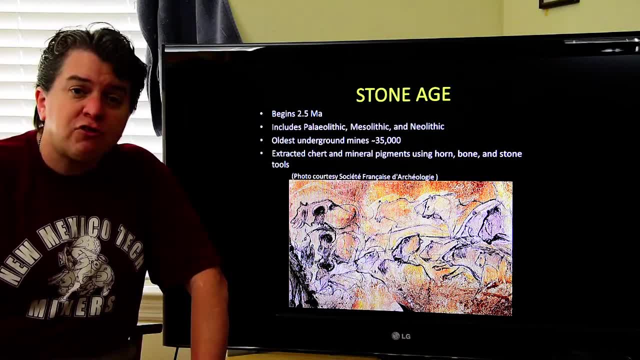 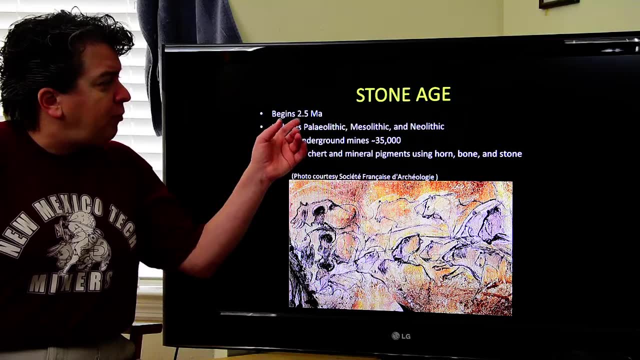 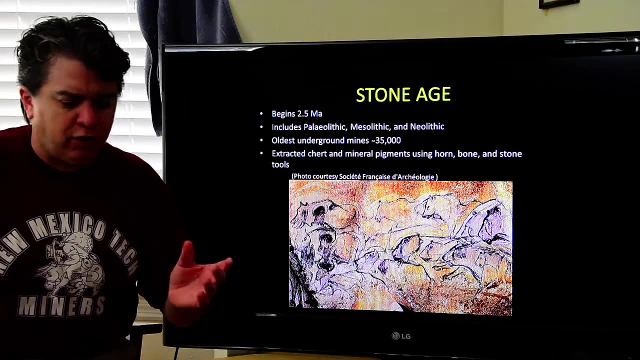 how our uses of minerals has changed over time And we're going to start all the way back in the Stone Age, And this begins about 2.5 million years ago. And one thing I do want you guys to realize: when we talk about these ages- the Stone Age, the Bronze Age, the Iron Age and all 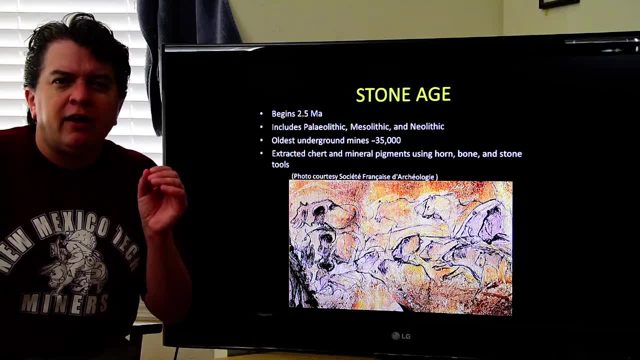 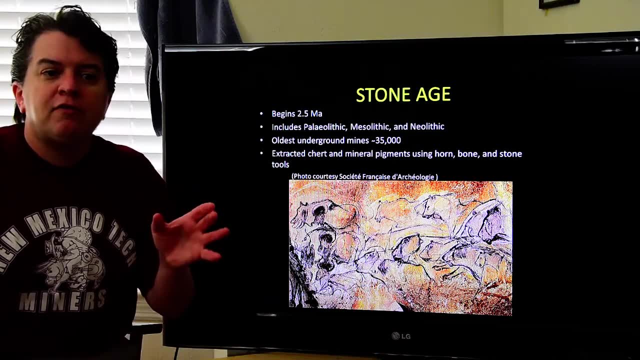 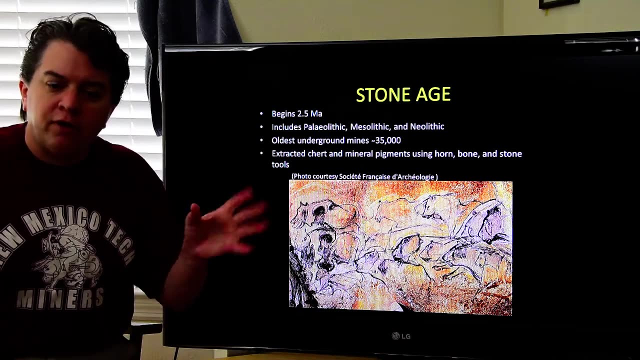 that kinds of stuff, those things. they're not exactly time periods, They're more like steps of technological development. So the Iron Age begins at different times in different places. So the numbers that I'm going to give you here are kind of estimates. So we have the Stone Age and this.